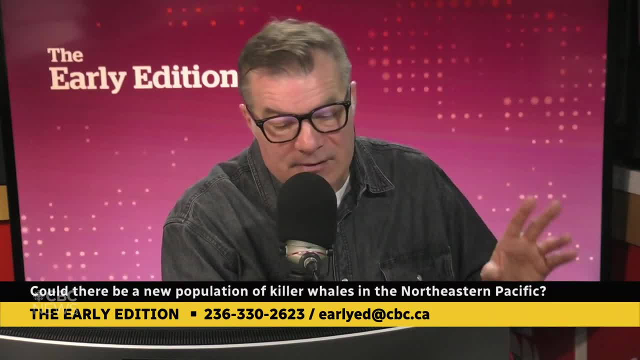 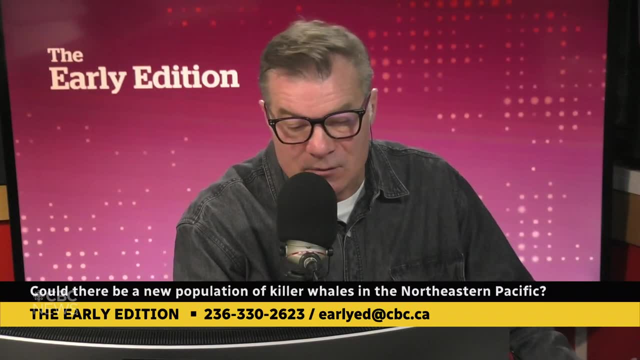 And they believe that 49 orcas could belong to a subpopulation of transient killer whales or a unique oceanic population. And joining us now is UBC professor of zoology Andrew Treitz is with us. He's co-authored a study with seven others looking at this group of orcas. 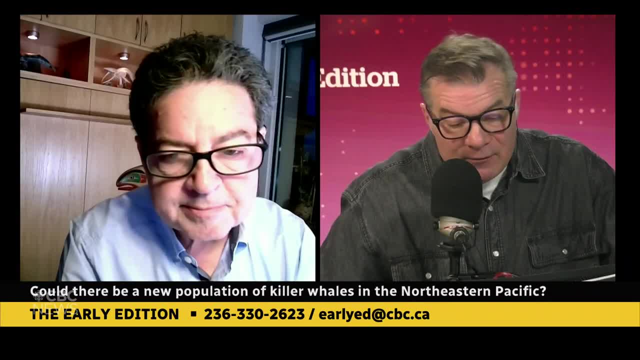 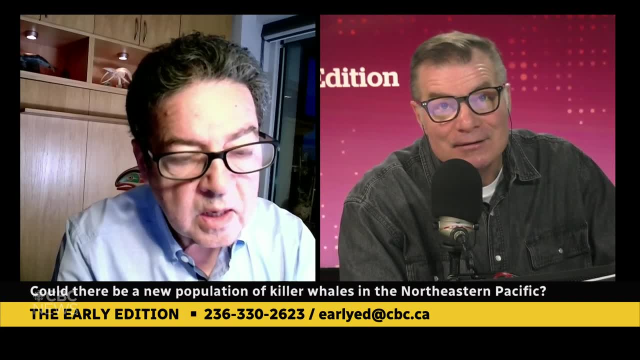 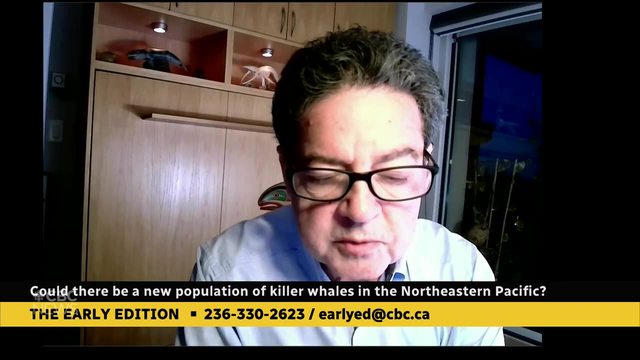 Good morning to you. Good morning Andrew. just how groundbreaking- or, I guess, how ocean-shaking- is this study. I think each time someone goes out to the open ocean, looks out and discovers something that we hadn't noticed before, I think each one of those is groundbreaking. 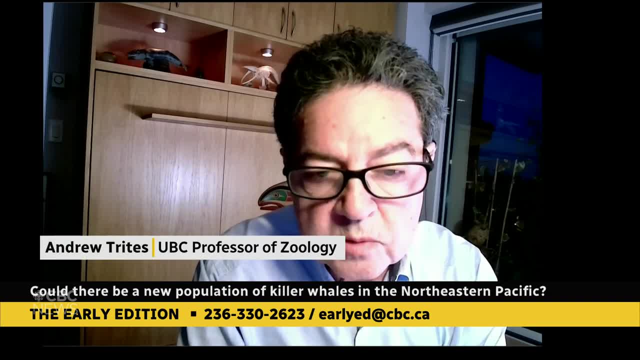 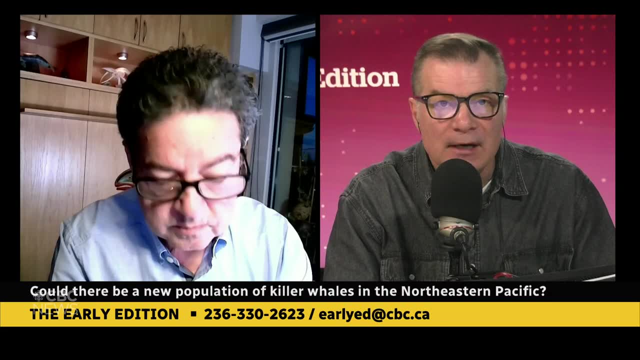 It makes us aware that there's more out there than what we have ever truly appreciated. All right, And so what have we been able? I mean, first of all, we're talking about 49 individuals in this. Is that right? We're up to 49.. 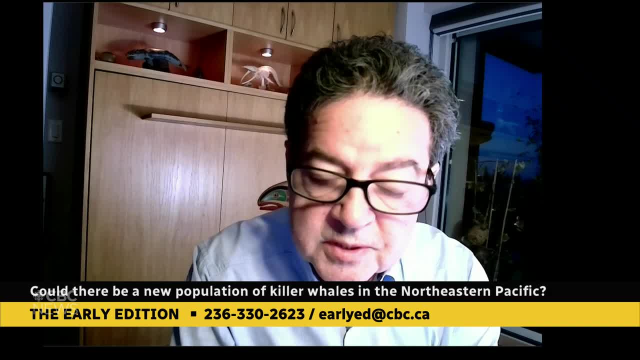 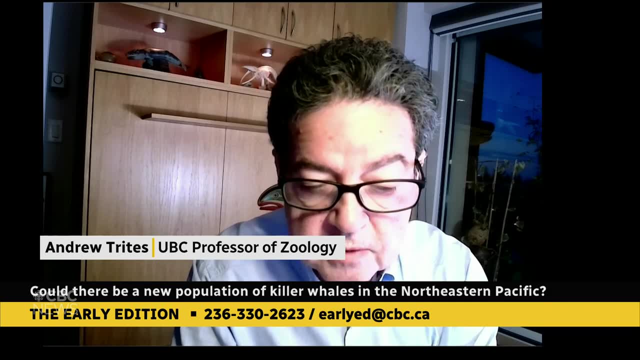 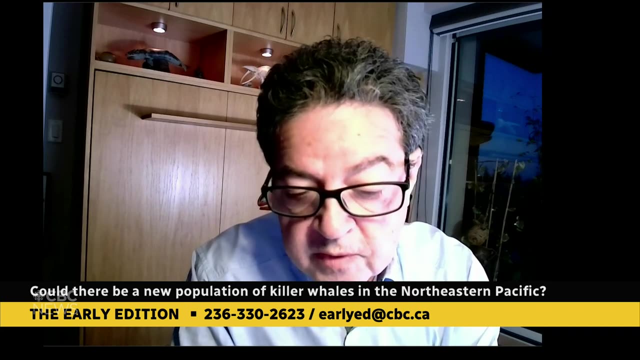 But, like with all of these newly discovered populations, as more pictures come in, the numbers will go up until eventually hits a plateau. And so, since we put this together, we have heard and have become aware of a few more individuals. We don't know where it's going to top off at, but it could well be 100, or perhaps even 200. 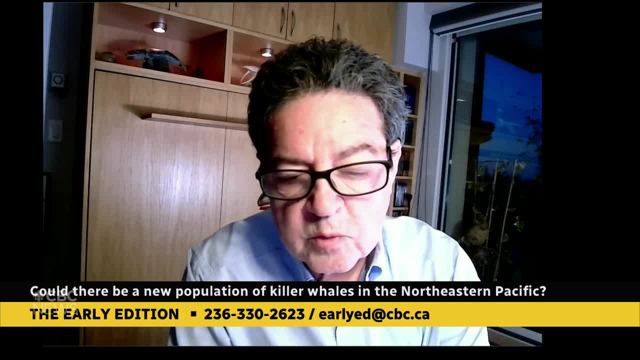 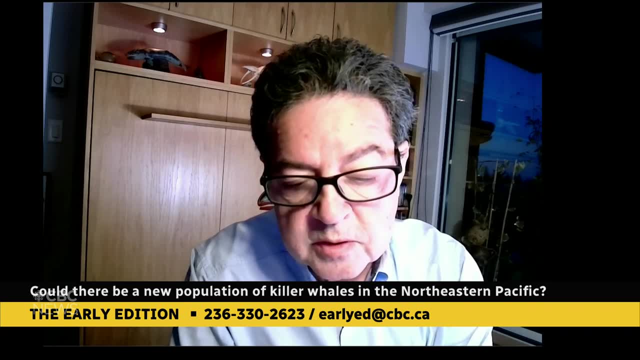 The problem is that it's so far offshore that very few researchers ever go there, And if people have gone out and seen killer whales, they probably haven't been equipped with cameras to turn in pictures. We're hoping that, by putting this out and making people aware that every picture is helpful, 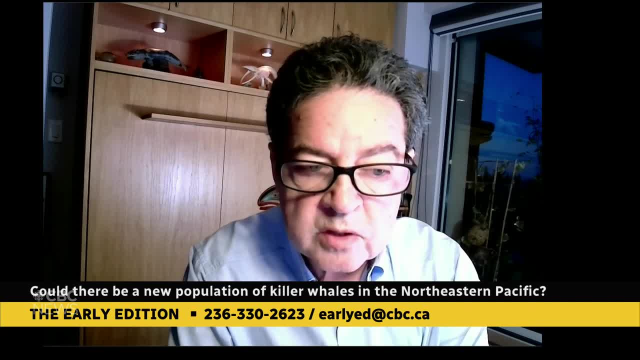 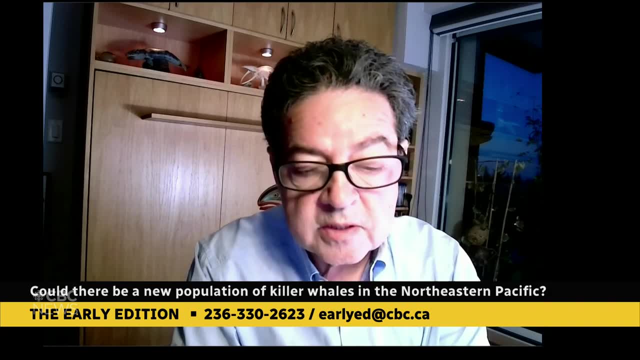 and particularly if you're out in bodies of water where very few people go- and that's true here in BC as well- we have very few opportunities to go way, way, way offshore to see exactly what's there. Well, and that's what I'm curious about, because we're curious about, rather, you know, we said California and Oregon- 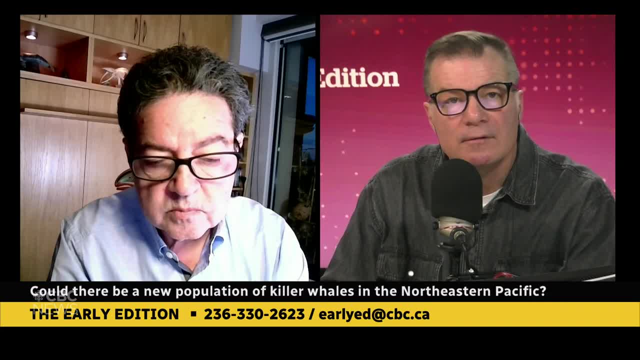 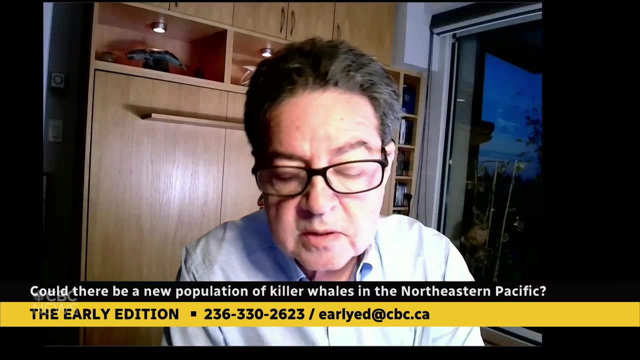 Are they coming as far north as offshore? Are they coming as far offshore of British Columbia? Who knows? It's possible They may well be restricted further south, But you know, I'd say that you know, with killer whales it's a species that fascinates the entire world. 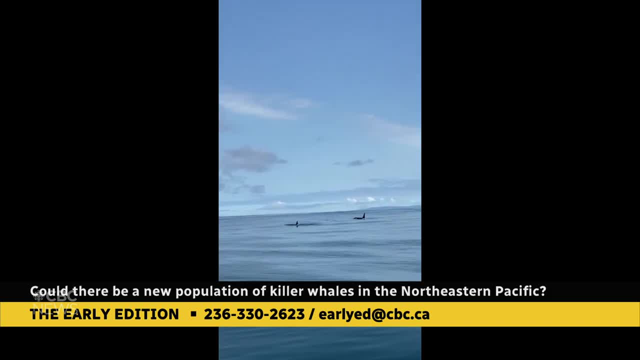 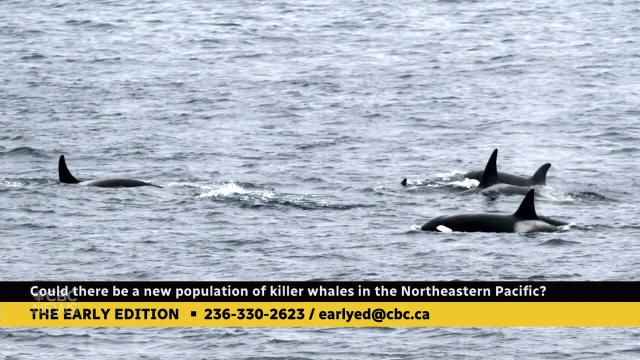 And it's in part because I think they share some of the characteristics that we do in terms of some of the family groupings, the bonds between mothers and calves, social structures, movements, even some of the fussiness they have in terms of their diets.